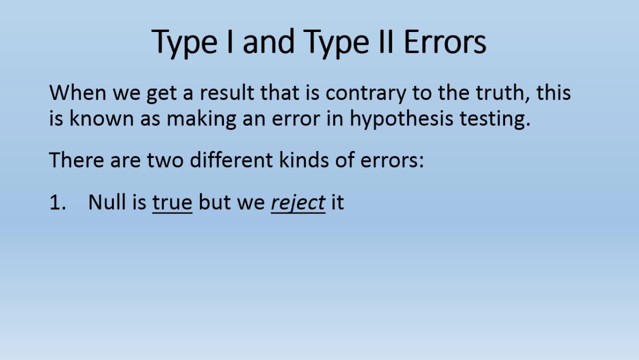 We have the error where the null is true but we reject it based on our test. and then we have the other kind of error where the null is false but we accept it or, using the other language, fail to reject based on the results of our test. 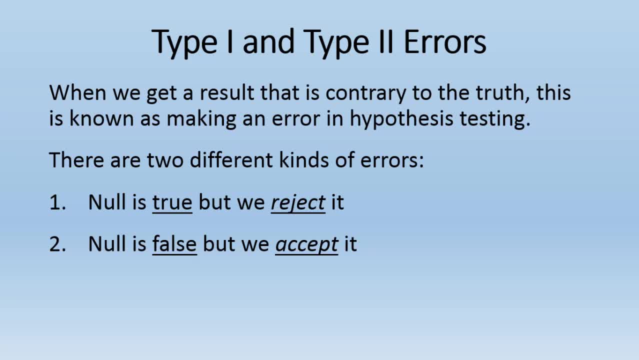 Now you should take a moment to look at this and make sure that you can see the inconsistency in these two statements: If the null is true, we reject it. that's an error or a mistake- and if the null is false, we accept it. 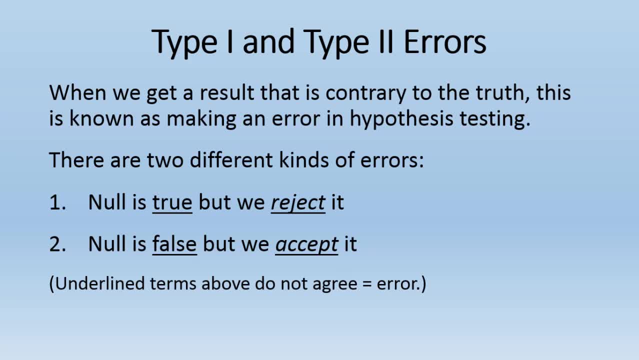 that's also an error or a mistake, And these terms do not agree, as I just said. so that's why we have errors here. So whenever this happens, we have made an error if we do either one or two. There are also two types of correct decisions in hypothesis testing. 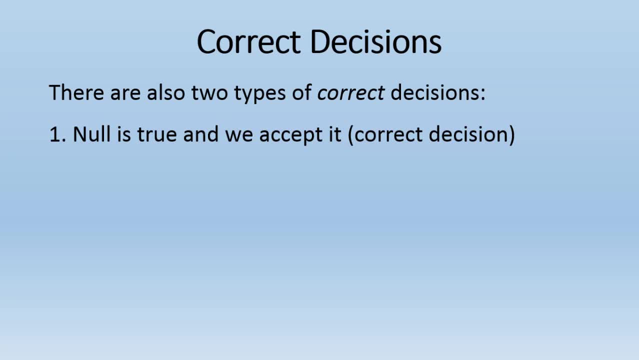 The first one is the null is true and we accept it. So if you think about that, if the null is true and from our test we accept it, then we've made a correct decision there, so that's good. And then the other scenario is where the null is false and we reject it. 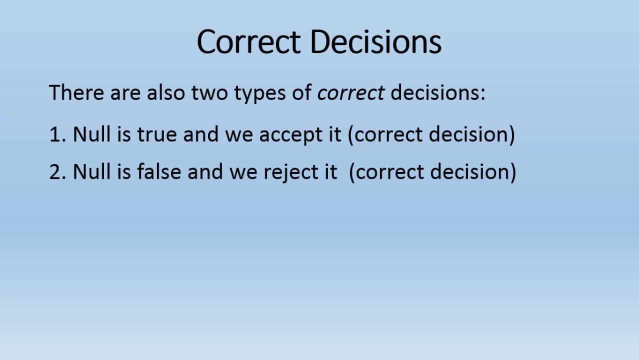 based on our data, So that's also a correct decision. While these are the two types of possible correct outcomes in hypothesis testing, let's take a closer look at the two different types of errors that can be made- those two we looked at previously. We'll examine those more closely next. 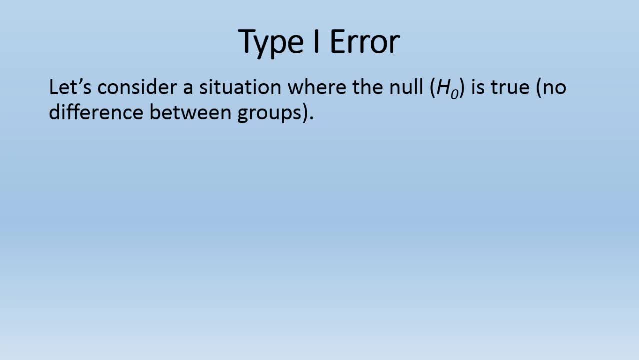 So let's consider a situation where the null is true, where there's really no difference between the groups And, to make this a little more concrete, assume that we're looking at the first-year collegiate experience in males and females Perception towards college: how much they feel like. 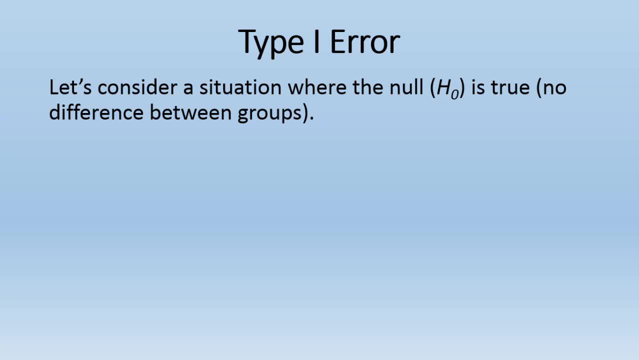 they're part of the experience at the University And let's say, for the purpose of this example, that it's known that males and females really there's no difference between themselves how cohesive or how much they feel like they're part of the University on average. 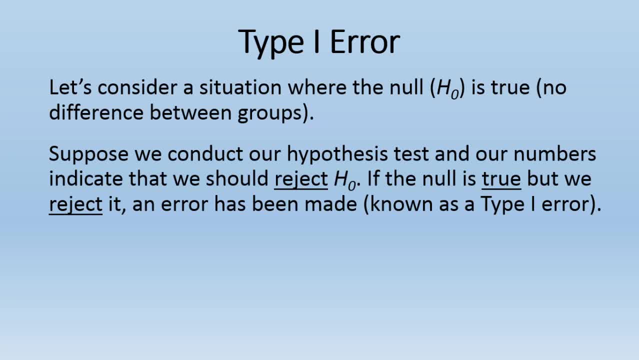 Just assume that, for this example, Let's say that we conduct our hypothesis test and our numbers are true. our numbers indicate that we should reject the null. So, with our example, let's suppose that females in our study that we did, indicated that they felt more connected or engaged in the